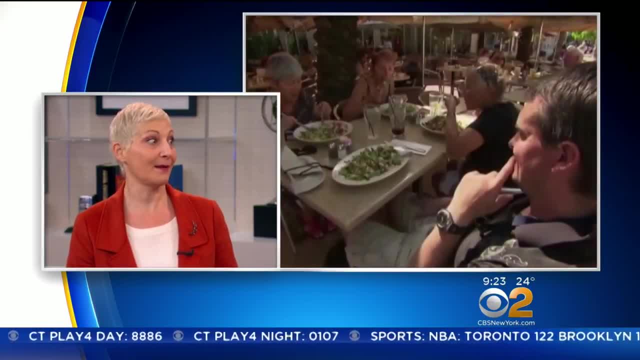 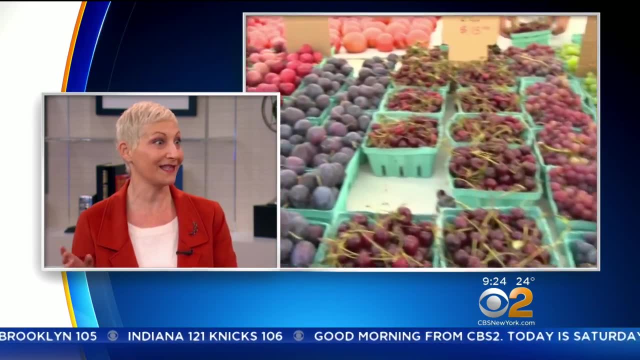 but it's also about talking about that food like it's yummy, right, Because we often say like, oh, eat this because it's got vitamins. And then we abdicate all those great words to the brownies: Oh, it's yummy, and crunchy and creamy or whatever. So we have to start thinking about those. 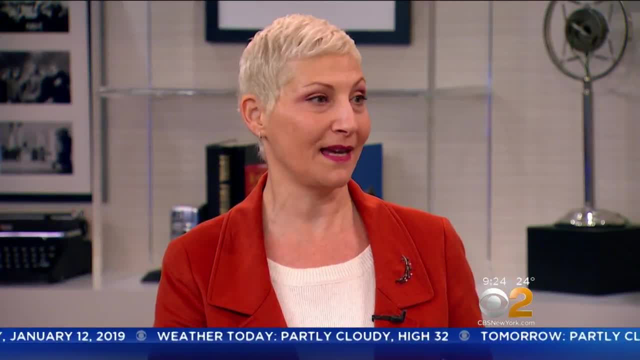 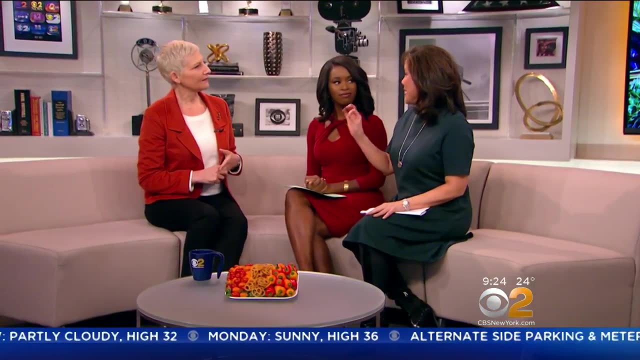 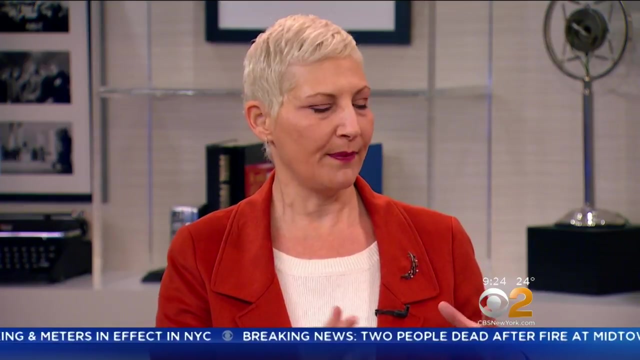 foods as yummy. That's a really big thing. Well, I also have found that you came up with like different acronyms to kind of remember things like MVP. Let's start with P being proportion, Proportion. That's right. You want to start making sure that your diet is in the 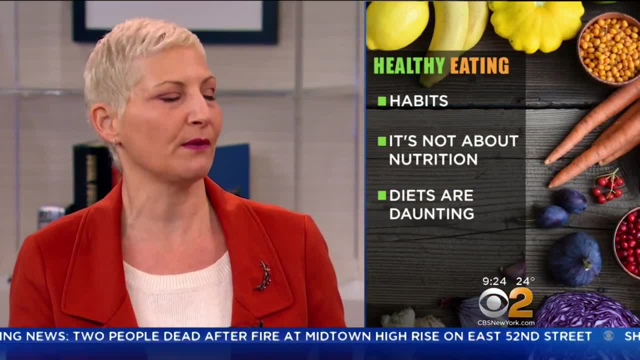 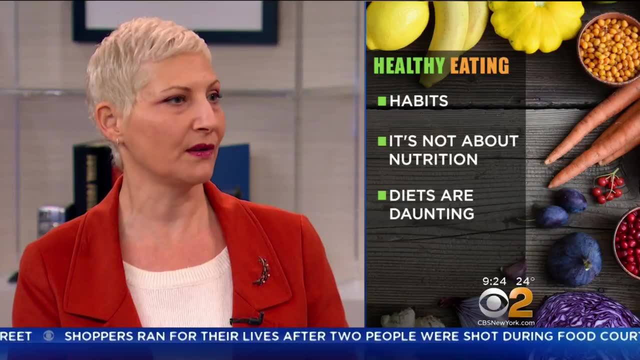 right ratio. So we're eating the healthiest foods the most frequently, And that doesn't mean that you can't eat the bad foods, right? You just have to put them in the diet in the right ratios, And so that's a big picture. 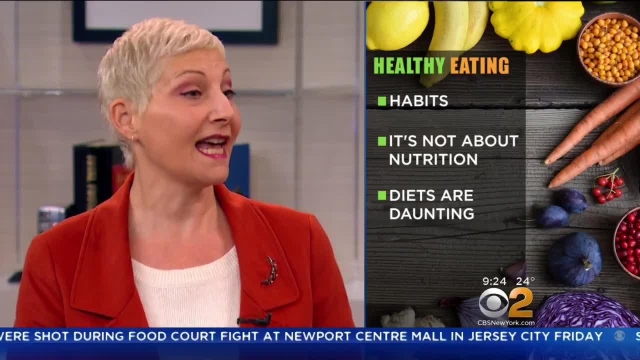 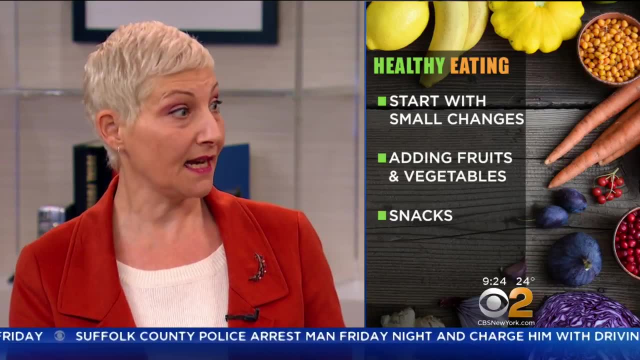 That's a big thing that we need to think about. V is, of course, variety. right, We want to make sure that we're eating different foods from day to day, But the one thing I want to say about changing your healthy eating habits is that we need to think about what I call the happy bite. 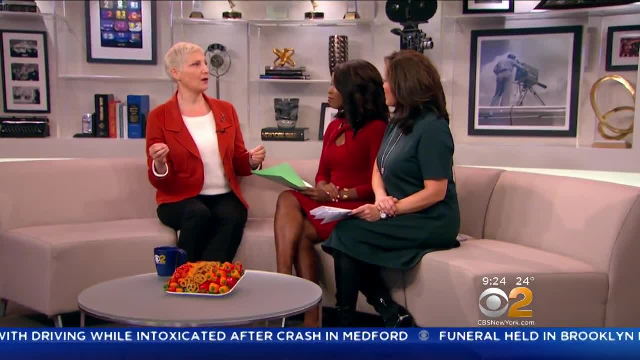 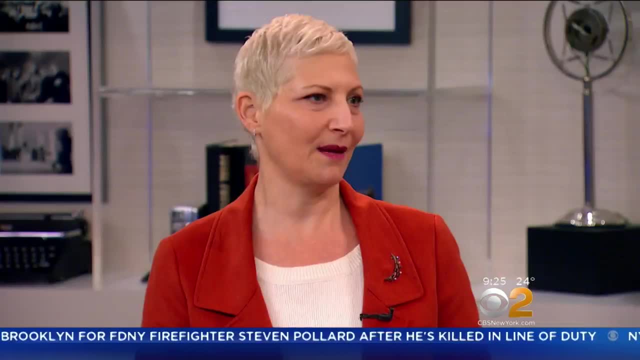 which is a couple of bites of fruits and vegetables spread out through the day, really adds up. You don't have to eat a huge portion if it's not your thing. And the final thing is moderation- right, Because moderation is really about portion size: eating when you're hungry and stopping when you're. 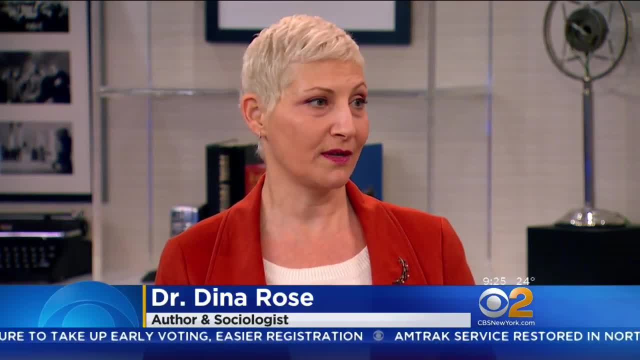 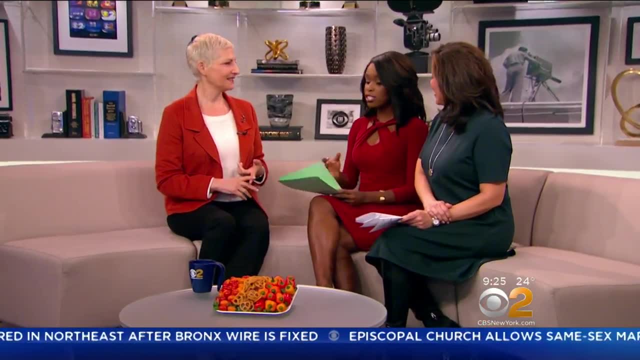 full. But that's also really about not eating because you're bored, sad or lonely, right? We've got to get that emotional eating out of the picture too, Right? And you say, starting small is really key, especially when including your kids. 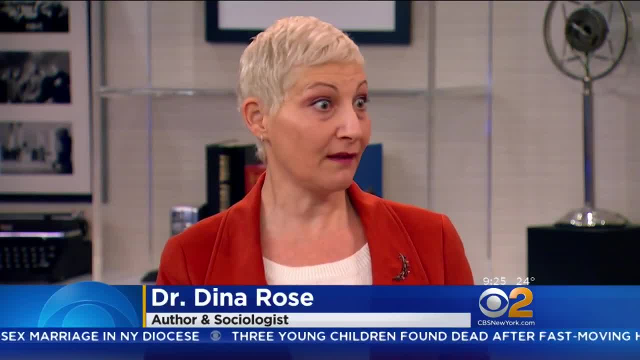 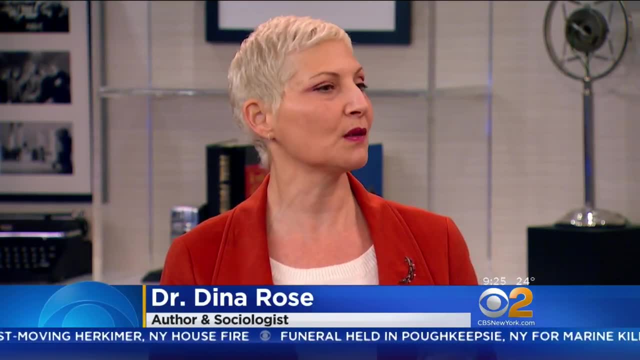 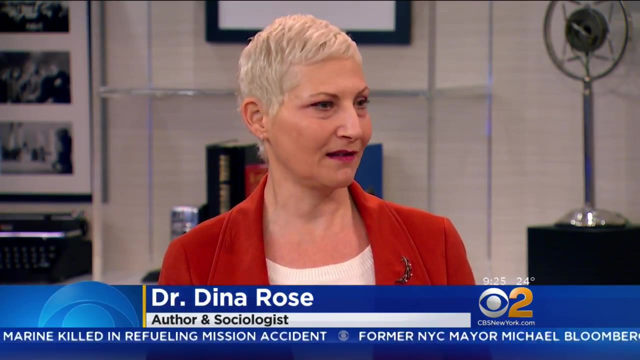 Right, It's exposing yourself and your kids to new flavors, new textures, new foods in very small increments to sort of just explore them. Because pressure here, pressure you feel yourself, pressure your kids, is the enemy right To the sort of just eat more, eat more. So small bites, small. 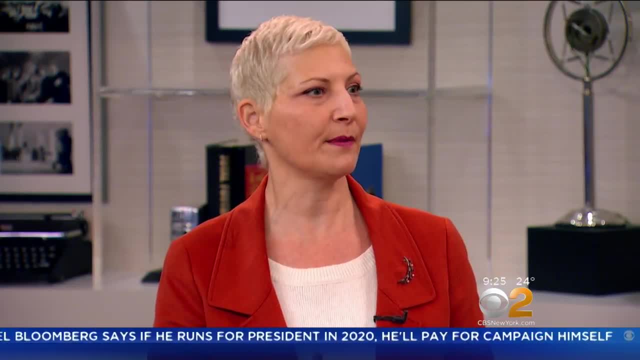 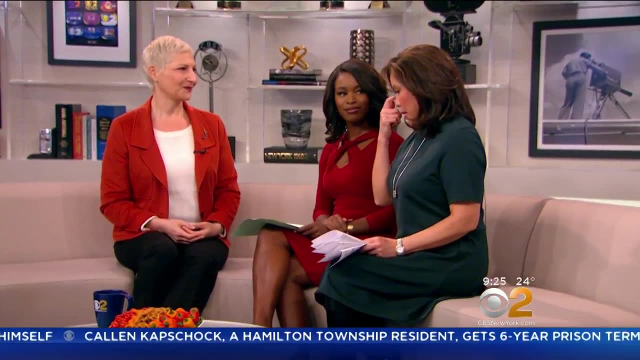 exposures, no pressure, change the mindset from thinking about nutrition to the habits, the big picture, And I'm guessing. one thing which is something I need to work on is to: if you want your children to eat healthy, you need to do the same, because they are always modeling the parents.